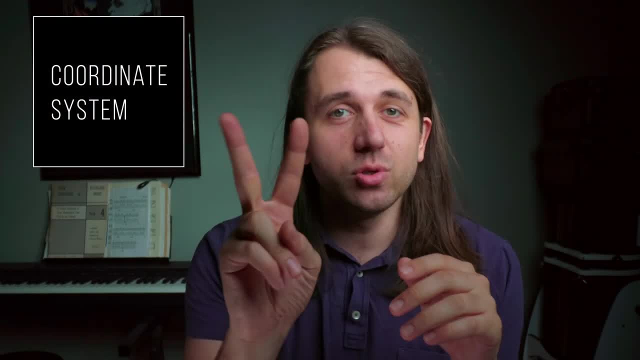 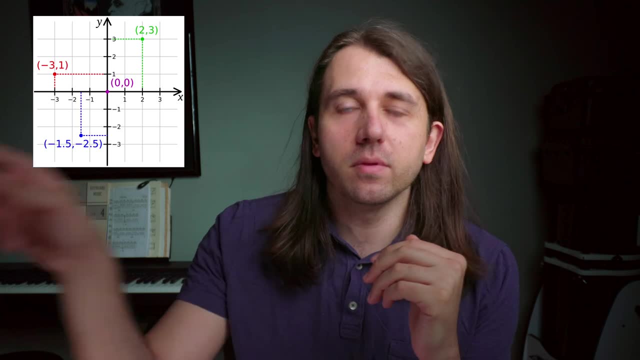 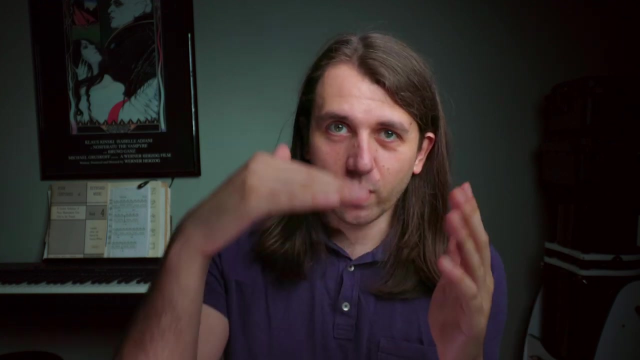 In a typical coordinate system you have at least two reference planes and then any location in that coordinate system can be explained as the distance from these two planes. So for example, for latitude and longitude, the two reference planes are the equator and the prime meridian. in Greenwich, England, Latitude is: 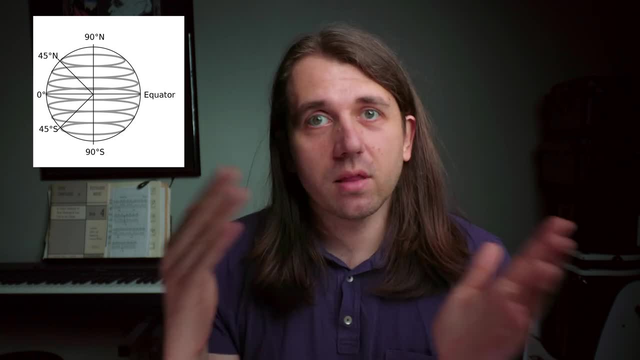 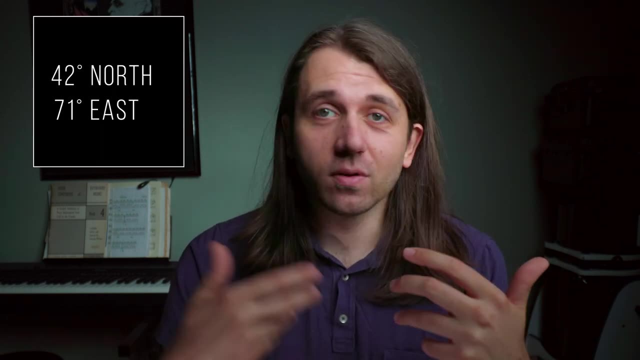 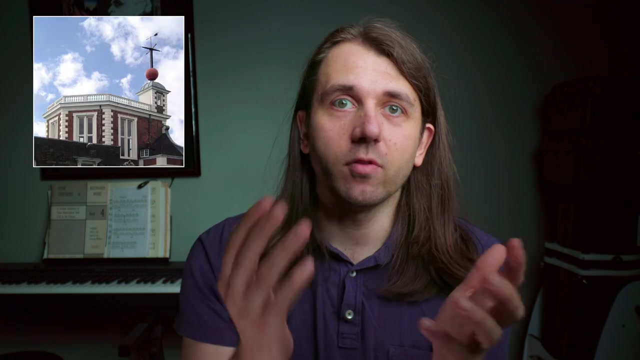 just your angular distance, either north or south from the equator, and longitude is your angular distance east or west from Greenwich. So when I say my coordinates right now are 42 degrees north by 71 degrees east, that means I'm 42 degrees north of the equator and 71 degrees east of the British Royal. 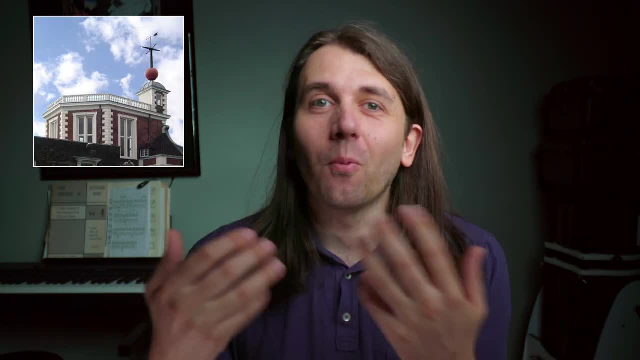 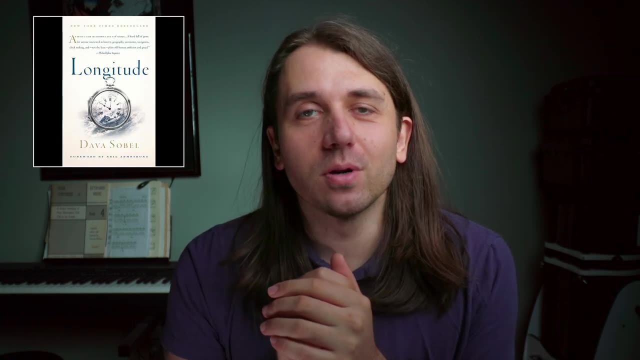 Observatory in Greenwich, England. Now you may have never considered why do we start measuring longitude from that specific place in Greenwich? I won't answer that in this video, but I will point you to a great book by Deva Sobel called Longitude for the whole story. 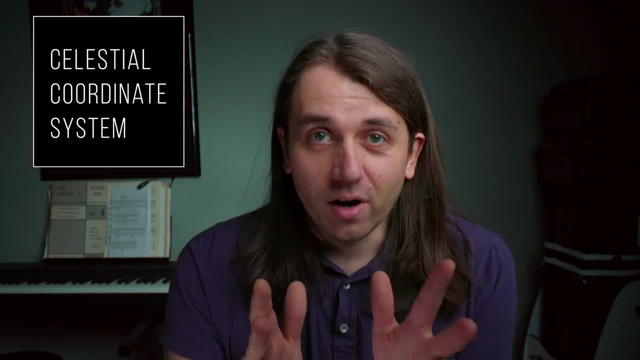 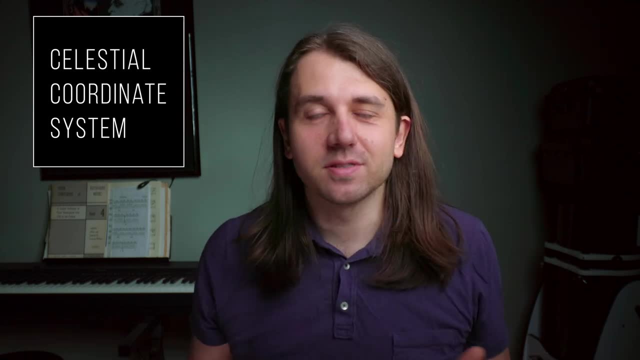 Now, if you're interested in learning more about longitude, let's go ahead and move on to the stars and what we call a celestial coordinate system. There are lots of possible reference planes for making a celestial coordinate system. One of the earliest used by ancient Greeks was the 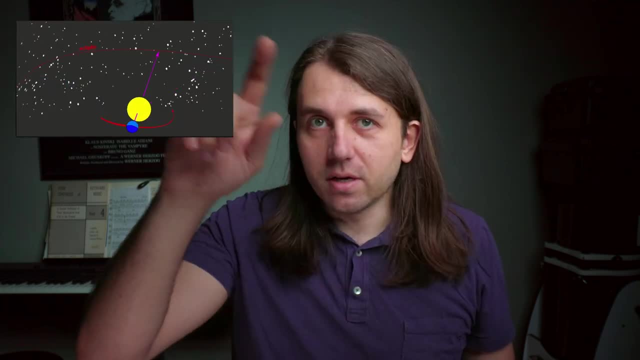 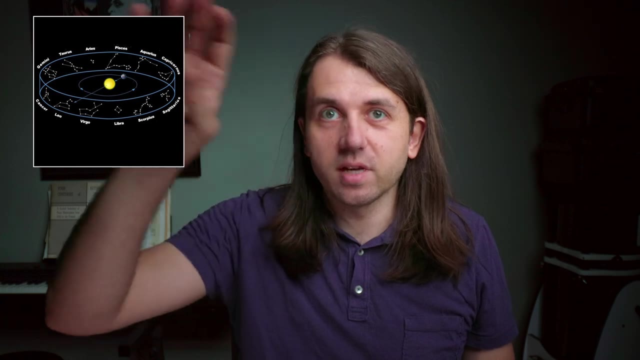 ecliptic, which is the path that the Sun appears to move through throughout the year in the sky. This is where the zodiac constellations come from. It's where the Sun is moving through those constellations in the night sky. You could make an ecliptical coordinate system, but the more common one. 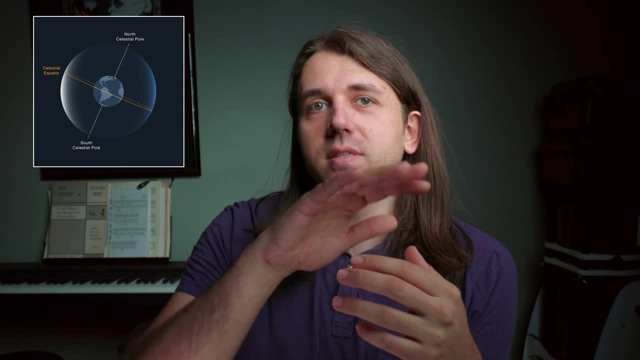 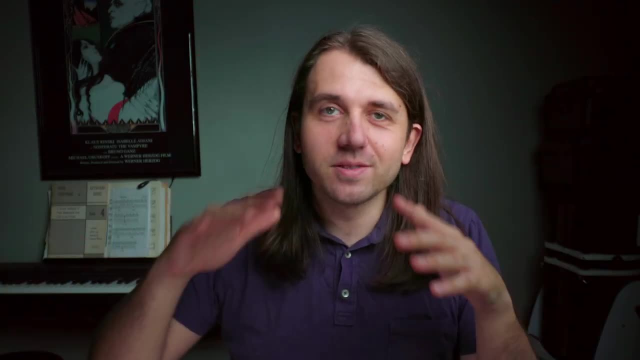 today is an equatorial coordinate system and, like the name suggests, this is based on the Earth's equator. Just imagine the Earth's equator extending out into space forever. The other reference plane other than the equator is a bit more complex. to wrap your head around, as it's both a time and a location. The reason it has to be both a time and a location is we're both rotating around our own axis, but also rotating around the Sun, which is why there are different constellations. 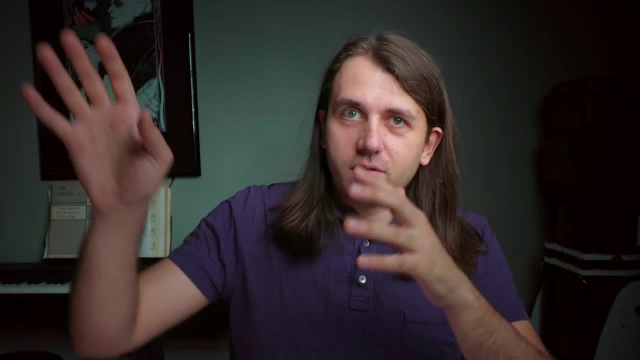 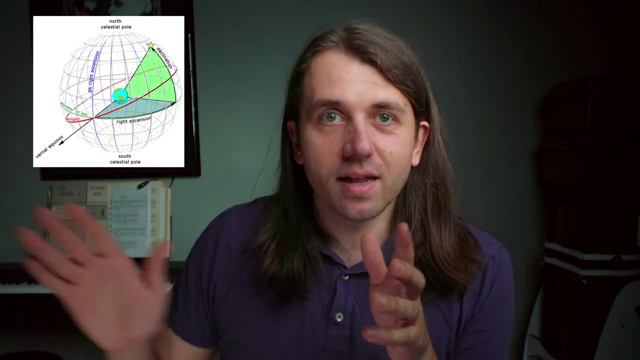 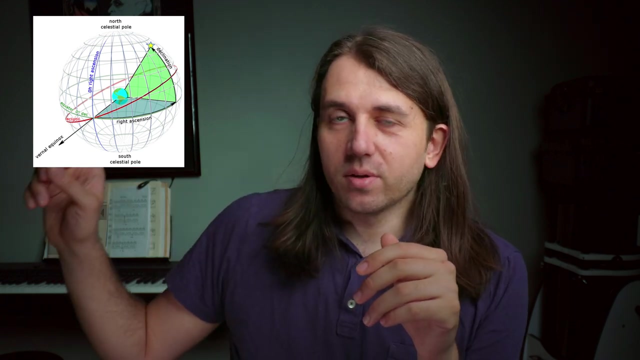 up in the summer compared to the winter, because we're literally changing where we are and facing a different part of the sun. The other reference plane is where the Sun is located in the night sky at the time of the vernal equinox in March. We then measure where the stars are located. 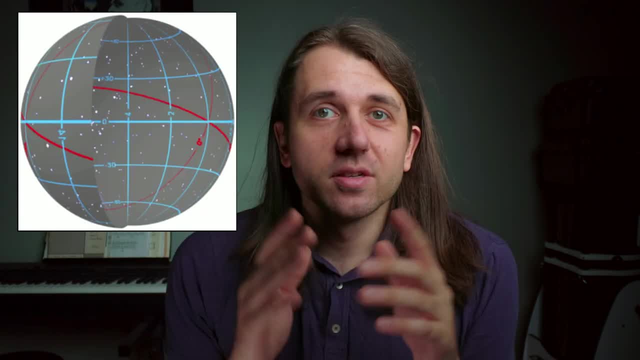 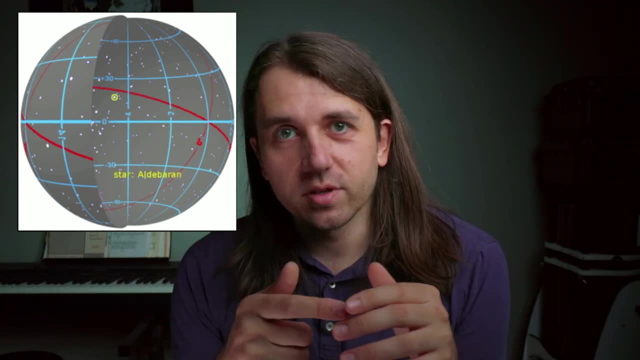 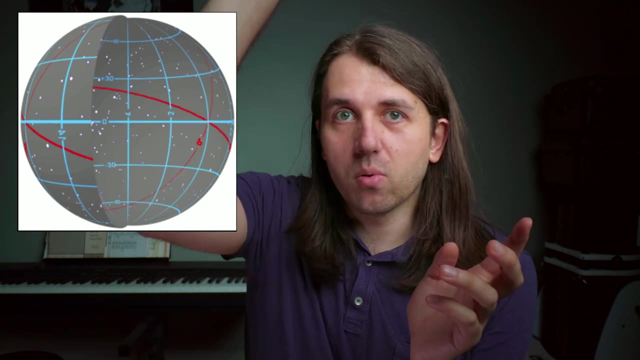 eastward from that plane and call this right ascension. To review, the two parts that make up equatorial coordinates for the night sky are: first right ascension, which is measured eastward from where the Sun is in the night sky on the vernal equinox, and then from that point, declination is how far. 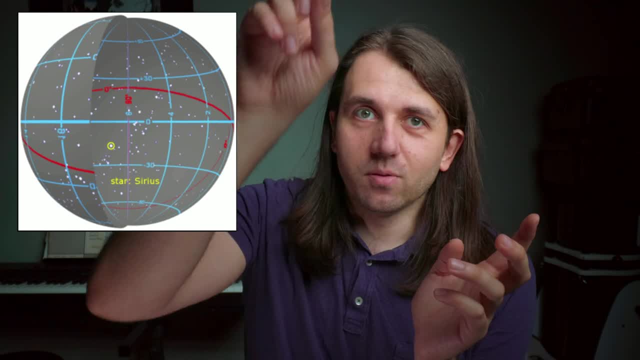 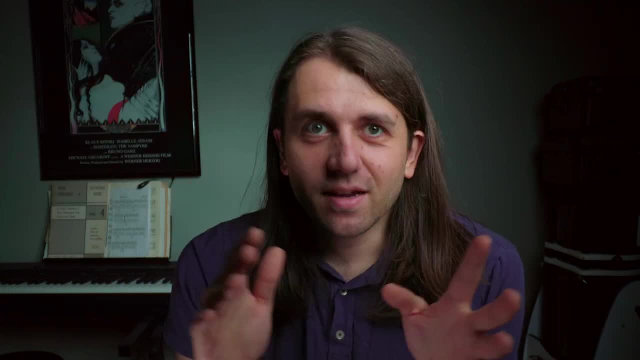 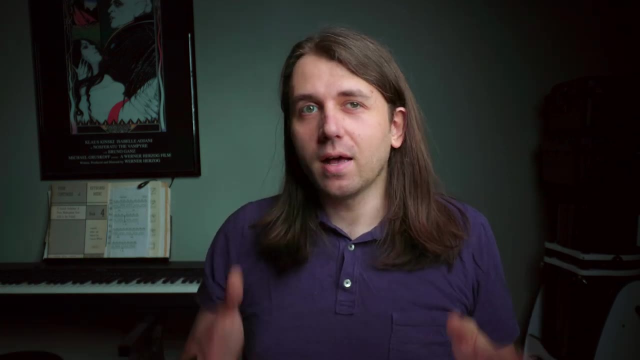 off from the equator. it is so up it would be positive degrees, down is negative degrees. the equator is zero degrees. now, to make this just a bit more confusing: declination, like latitude, is measured in degrees. right ascension could be measured in degrees, and sometimes is, but more commonly is. 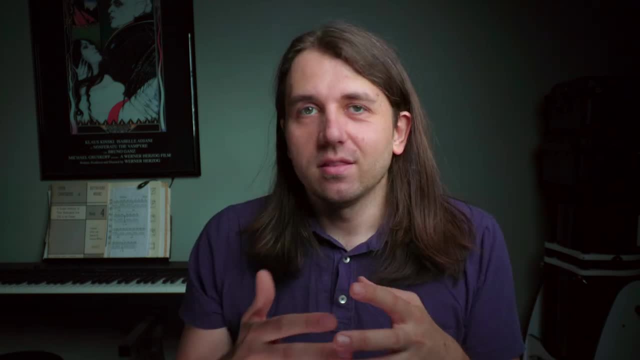 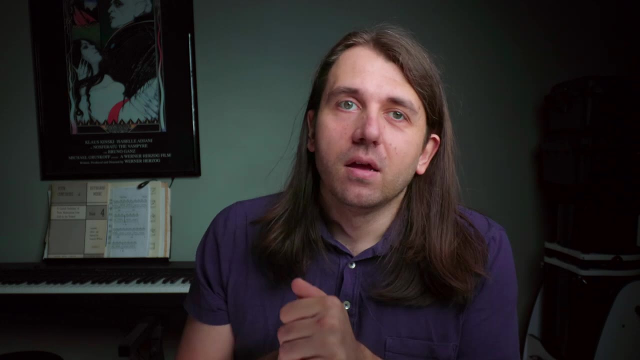 measured in hours, minutes and seconds. so instead of breaking the celestial sphere into 360 parts- that we would call degrees, we break it into 24 parts. we call hours, like a clock. Okay, so that's the equatorial coordinate system. you can use a star chart and what are called setting. 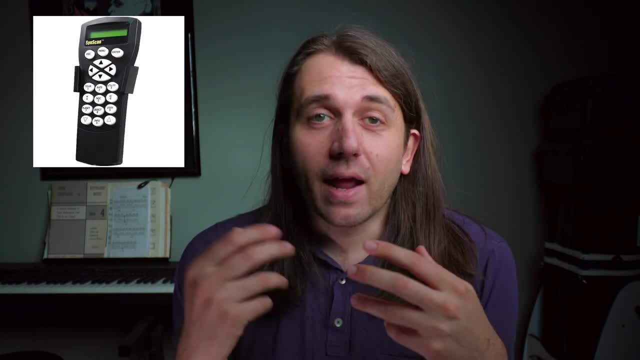 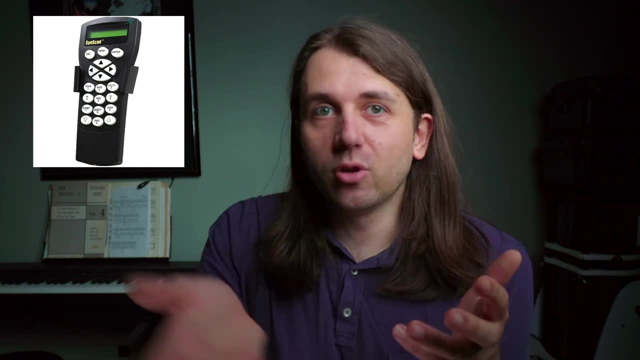 circles on an equatorial mount. if you want to go full manual, what I think of as GPS of equatorial mounts is a go-to system where you tell the system that's a computer, we're on earth, you are located in the precise time and date and 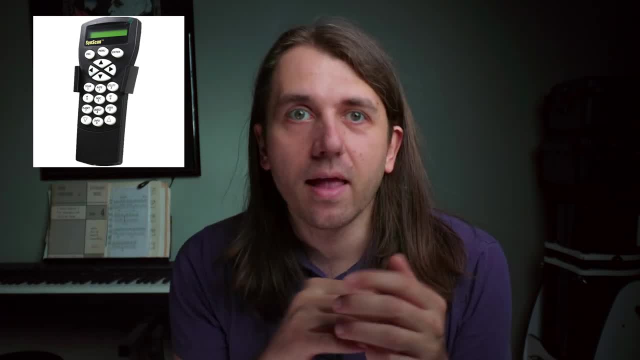 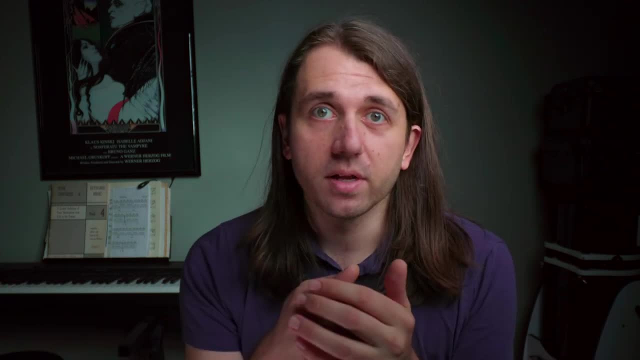 then it has a little database and it translates where the stars should be in the sky and automates the pointing of the telescope for you, based on these RA and DEC coordinates, which again are equatorial coordinates. but there's another kind of coordinate system we use all the time in astronomy, called a horizontal coordinate system. more 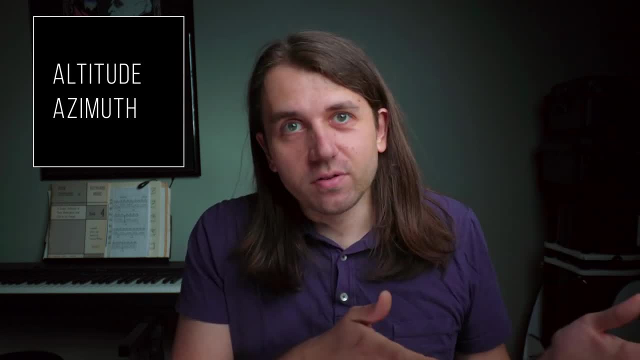 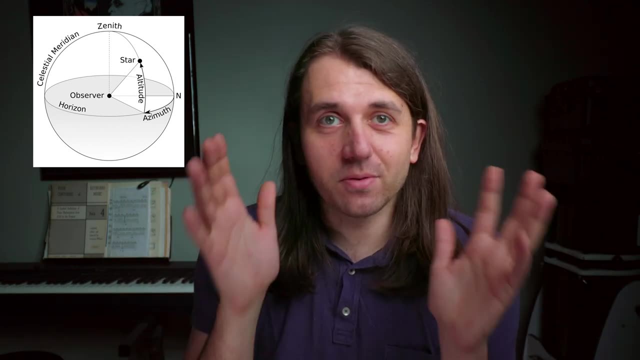 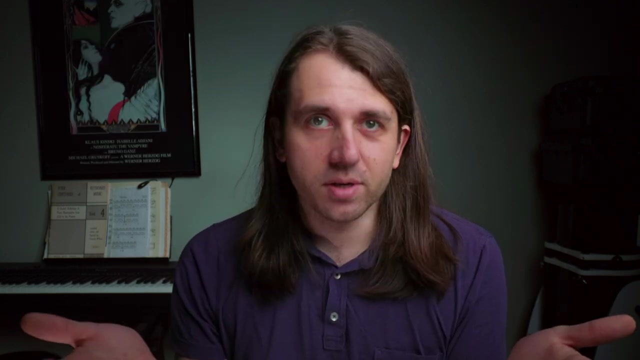 commonly known simply as alt as, which is short for altitude, and azimuth. with alt, as the two reference planes are north and the horizon at the actual time and location of where you're observing. it's called a horizontal coordinate system, but another way I think of it is just a local coordinate system. it's just for. 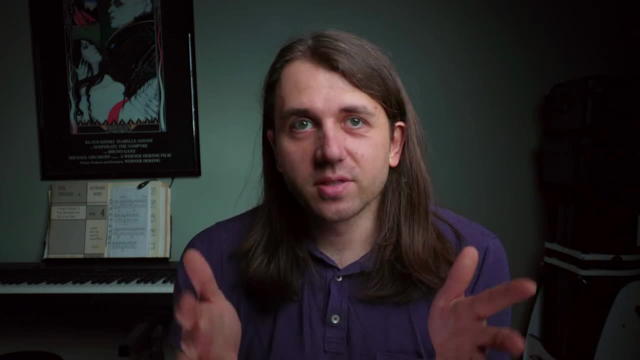 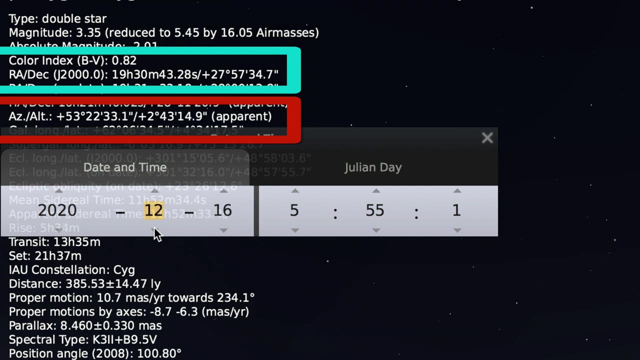 that moment, in that location, these coordinates, the alt as coordinates, don't really mean anything outside of that particular context. You can see if I change my time of day in stellarium the alt as keep changing while the RA and DEC stay consistent. but the reason we use alt as all the time is: 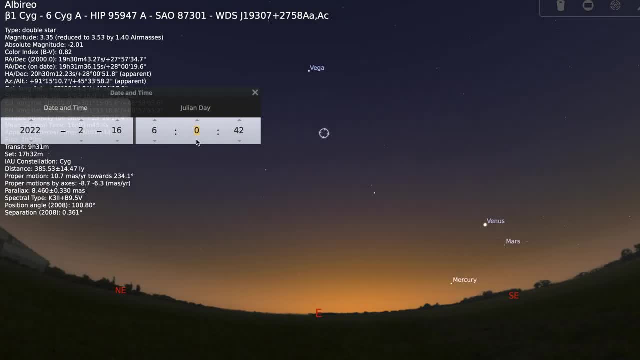 they're a lot more easy to understand. for instance, if I pull up alberio here and see the azimuth is 90 degrees, I know that's due east for that location, and if it's altitude is 45 degrees I know that's halfway up from the horizon to 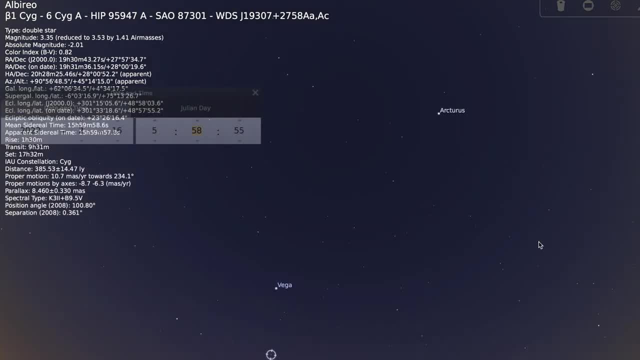 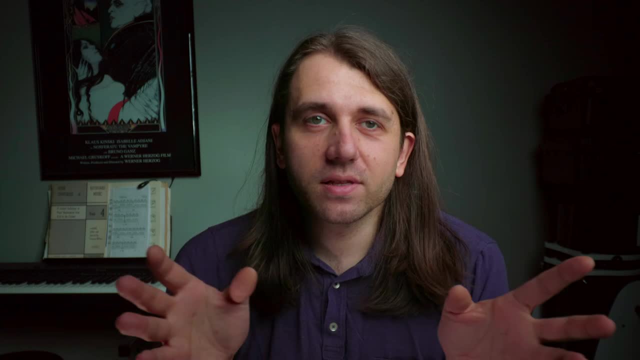 the zenith. the zenith just meaning straight up 90 degrees. now there are some fancy formulas for converting equatorial mounts. Now there are some fancy formulas for converting equatorial mounts. Now there are some fancy formulas for converting equatorial mounts coordinates to horizontal coordinates. but luckily we live in an age where all